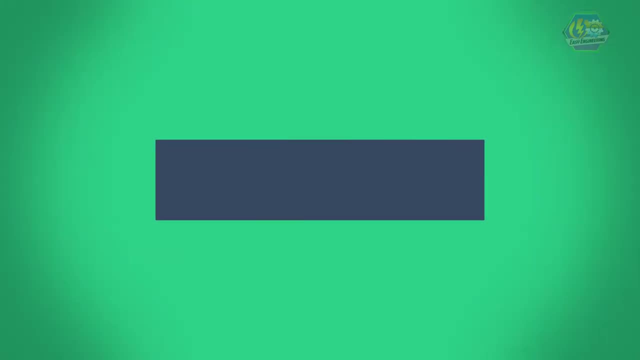 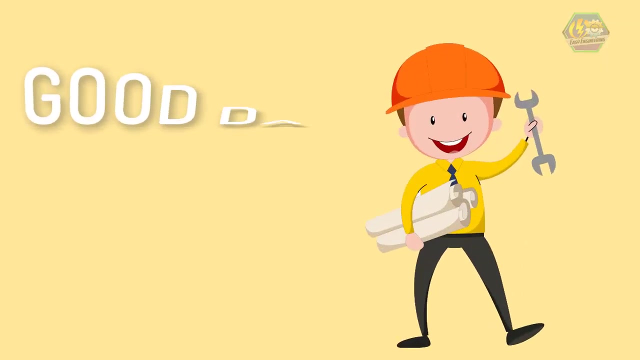 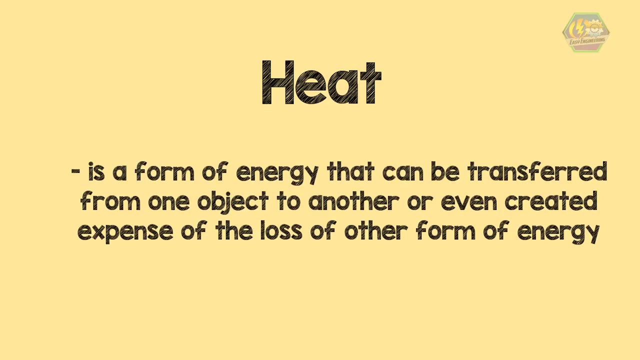 Good day learners. this is Easy Engineering. For today's topic, we are going to talk about heat transfer. Before we discuss heat transfer, let's define first heat. So what is heat? Heat is a form of energy that can be transferred from one object to another. 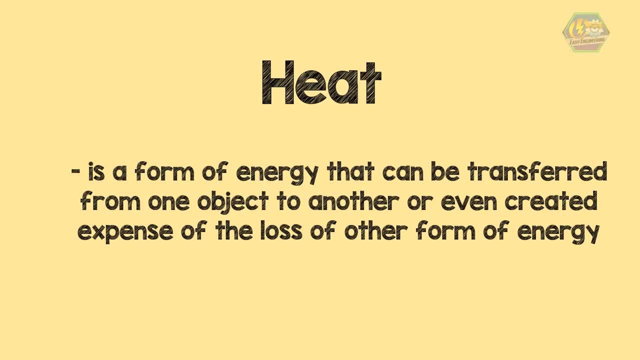 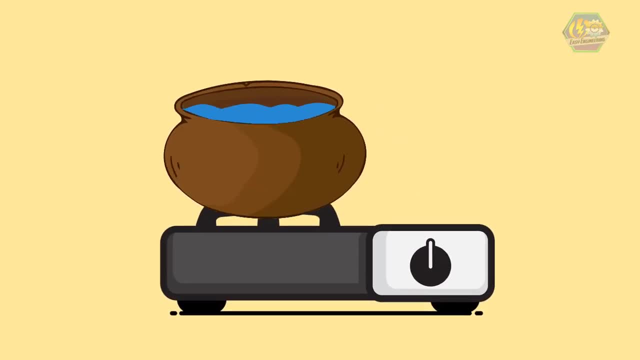 or even created at the expense of the loss of other form of energy. Now imagine you have a pot full of water and you put the pot on top of the stove. Now the pot becomes hot and, as the time goes by, the water began boiling. 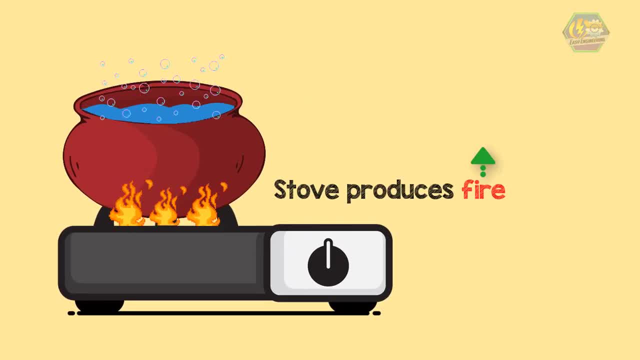 The stove produces fire, and the energy formed in the fire was then transferred to the pot. That's why the pot becomes hot and also because of that energy transfer, the water starts to boil. That process is called the heat transfer. There are three forms of heat transfer. 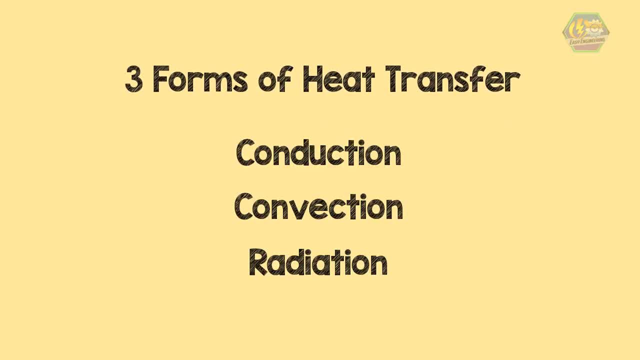 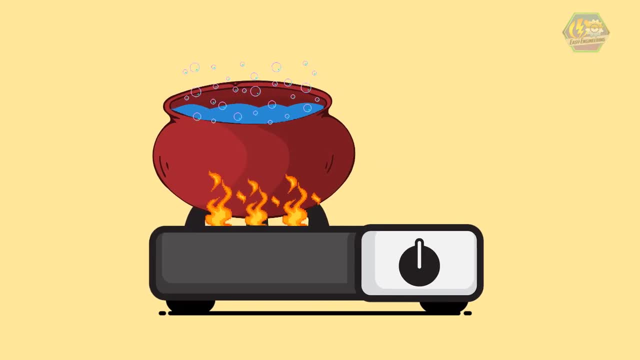 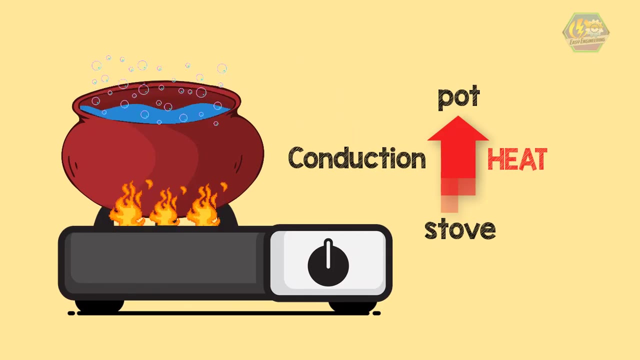 The conduction, convection and the radiation. When heating a pot full of water, all three forms of heat transfer are taking place. Conduction takes place with the transfer of heat from the stove to the pot. The water boils by the process of convection. 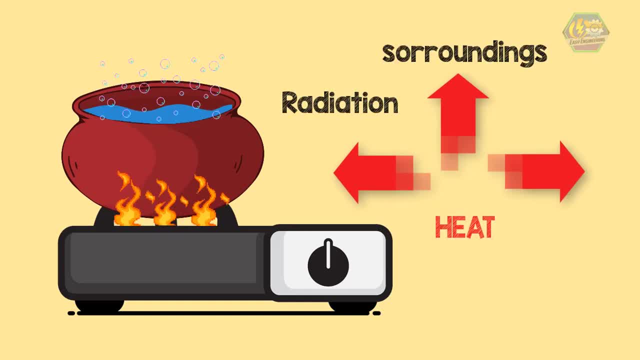 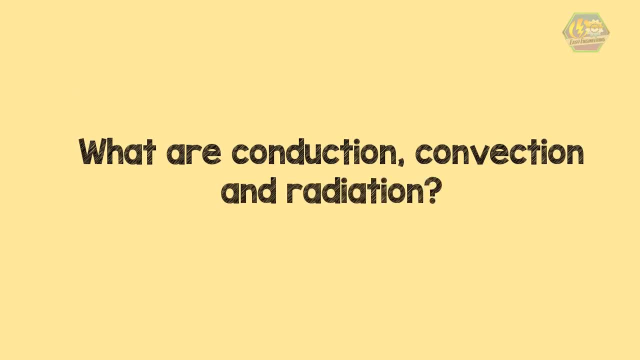 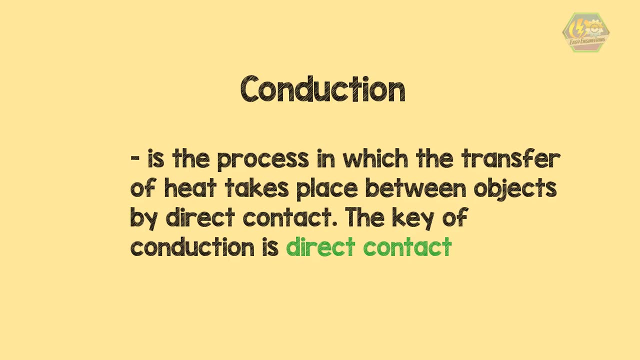 And the heat from the flame radiates to the pot. And the heat from the flame radiates in all directions. But what are conduction, convection and radiation? Let's discuss first the conduction. Conduction is the process in which the transfer of heat takes place between objects by direct contact. 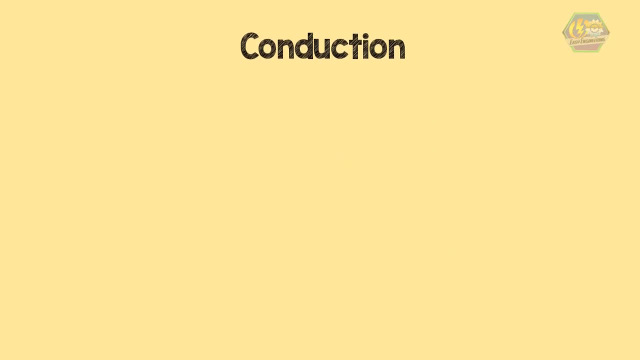 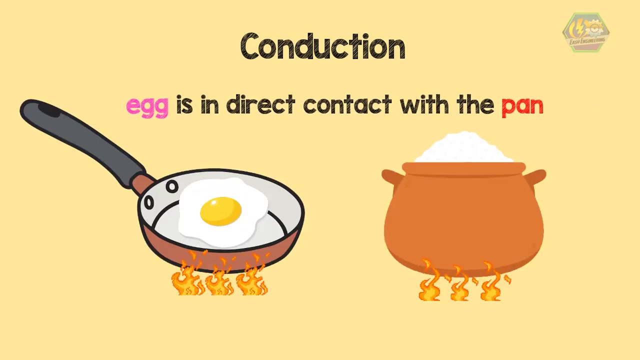 The key of conduction is direct contact. Notice that the pot is in direct contact with the fire. The energy from the pot to the egg is transferred in a process of conduction, as well as the energy of the pot to the rice. Notice that the egg is in direct contact with the pan and the rice is also in direct contact with the pot. 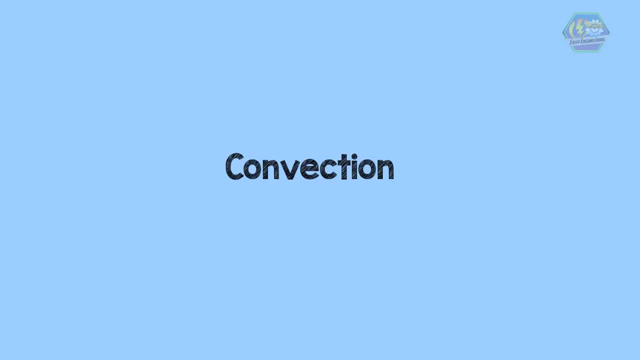 So now let's go to the convection. Convection is the transfer of heat by the movement of fluid. Hot beverages, or hot coffee to be specific, is another example of convection. You know why? It is because the steam coming out of hot coffee in the form of warm air rises.